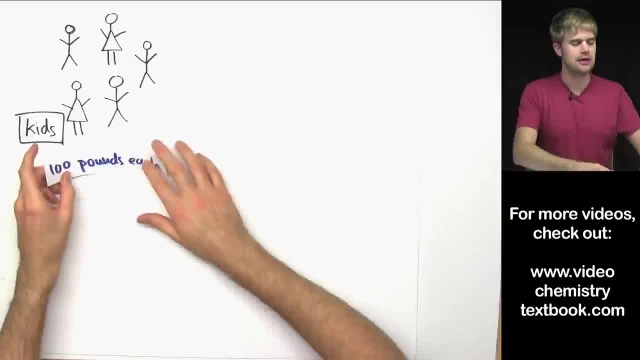 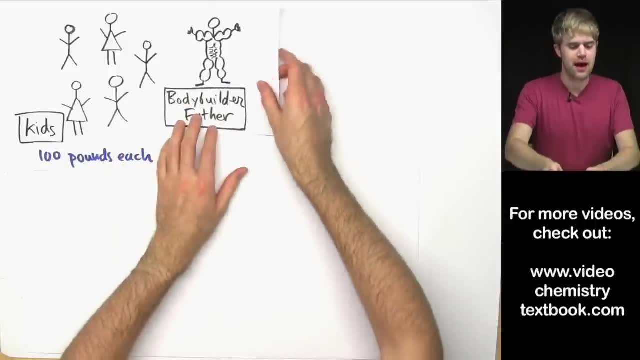 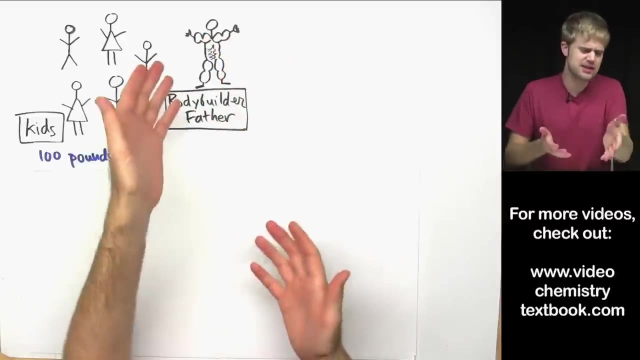 There are five kids, some boys and some girls, and, for simplicity's sake, let's just say that each one weighs 100 pounds. Now one of their fathers shows up and the father is a bodybuilder. Check out these muscles, Check out these eight-pack abs. I guess this means. 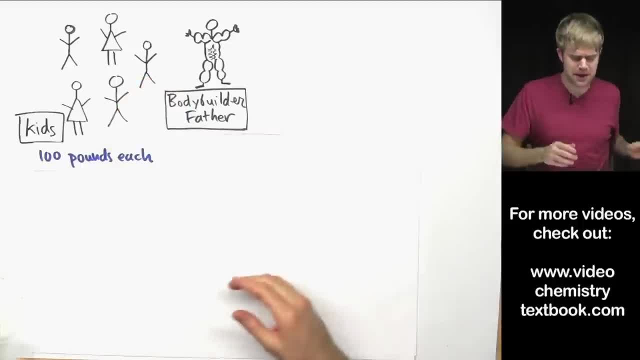 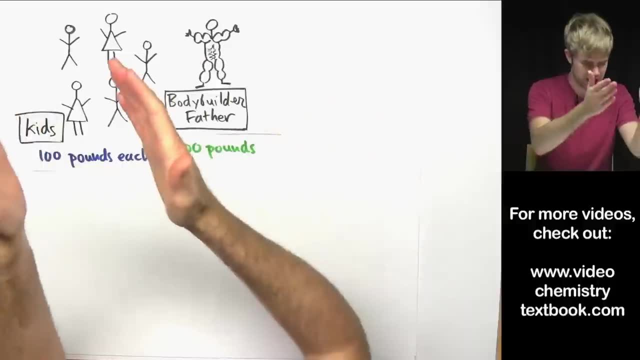 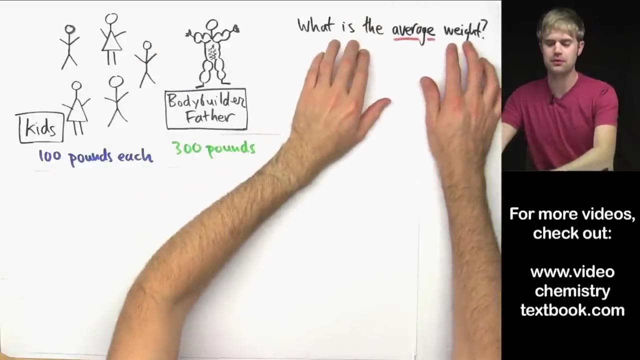 the guy has a shirt off, which is kind of creepy, but anyway, he's a big bodybuilder and he weighs 300 pounds. So now we have a group of six people here- The kids 100 pounds each and the father 300 pounds. So now you can ask a question about this group of people. 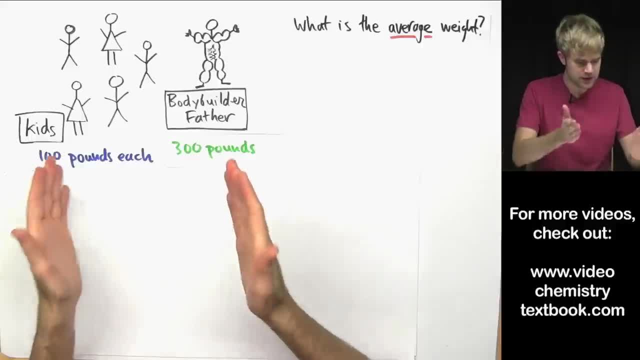 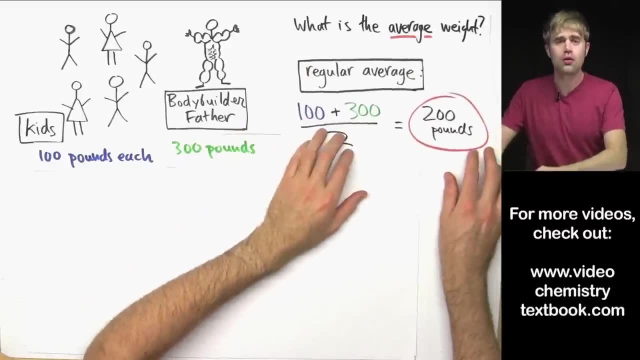 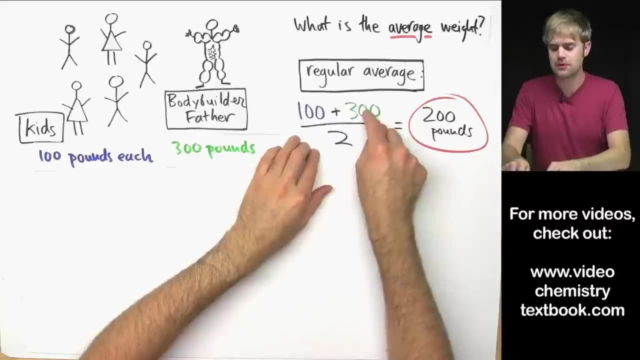 You could say what is the average weight? We've got these two different weights here: 100 pounds, 300 pounds. So you could calculate what I call a regular average. You take 100 pounds and 300 pounds because those are the two choices. You add them together and divide by two, because they're 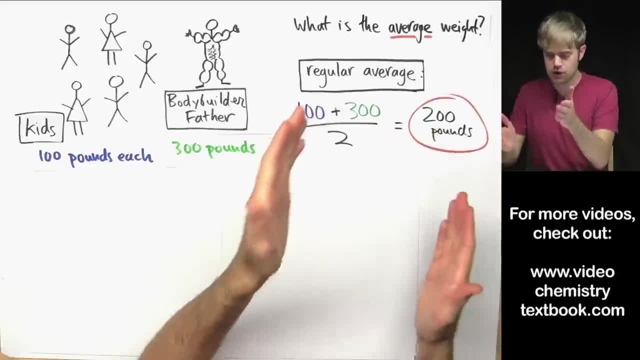 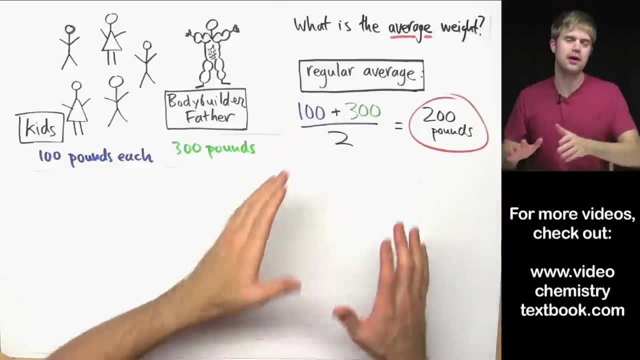 two different weights, You'd get 200 pounds, And 200 pounds is right smack dab in between 100 and 300.. So that's one way that you could get the average weight 200 pounds. But here's the thing, all right. 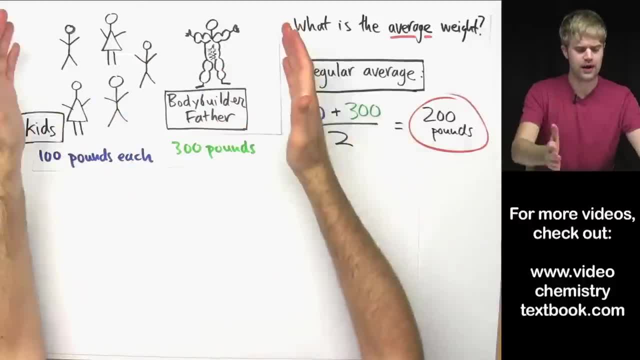 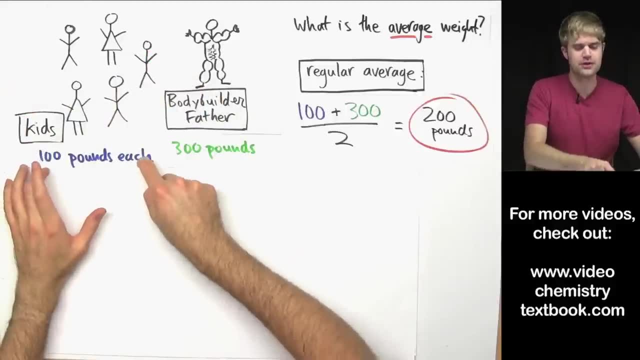 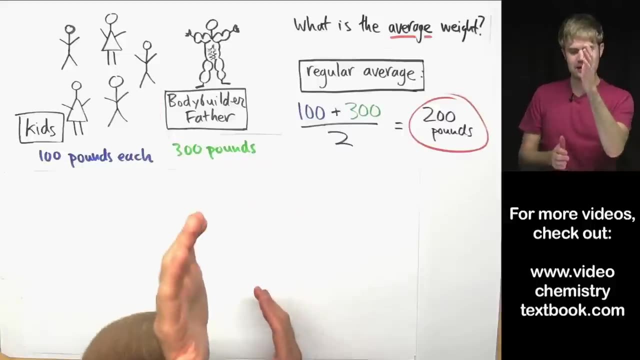 Is it really fair to say that the average weight of this group is 200 pounds, Because there are five kids that each weigh 100 pounds and there's only one father that weighs 300 pounds. So to say that the average weight is right between right in the middle of those. 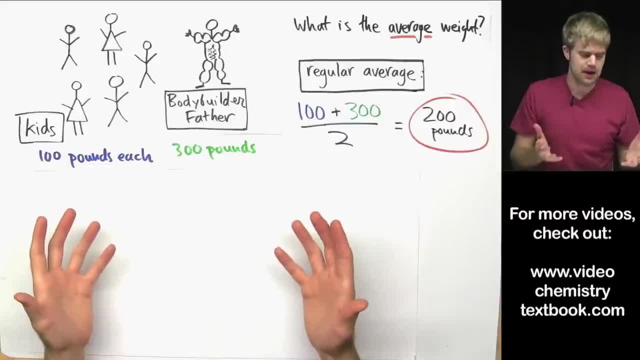 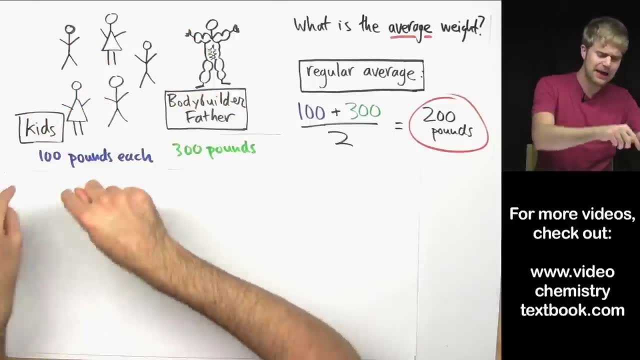 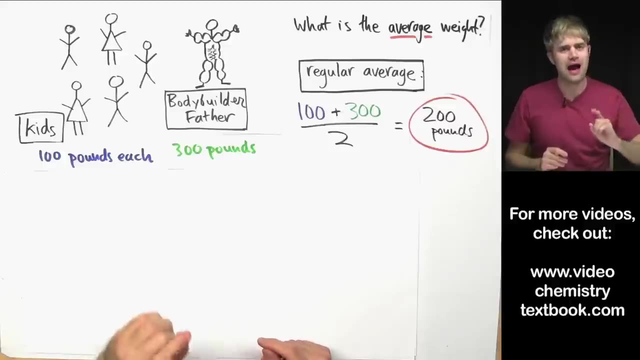 two weights kind of doesn't make a lot of sense. It feels like we should be able to take into account the fact that there are many more kids Who weigh 100 pounds, who weigh a lot less than the one bodybuilder father. This is where the idea of a weighted average comes into play. 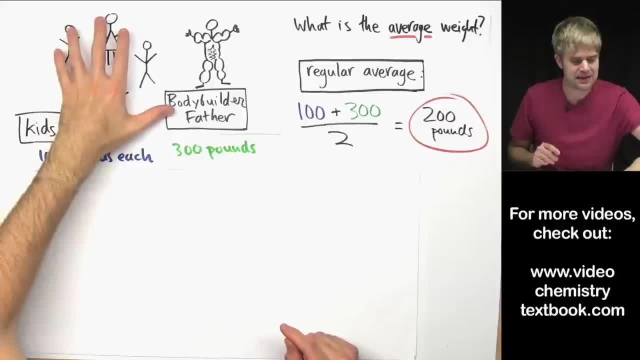 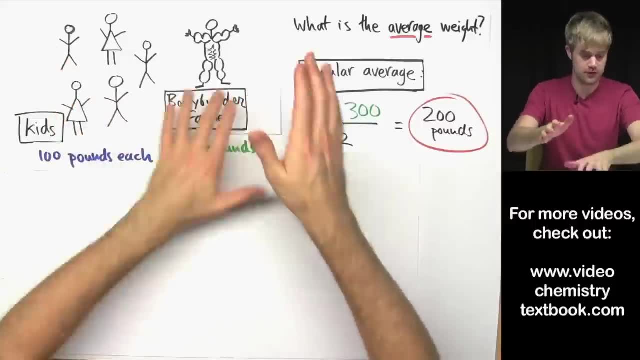 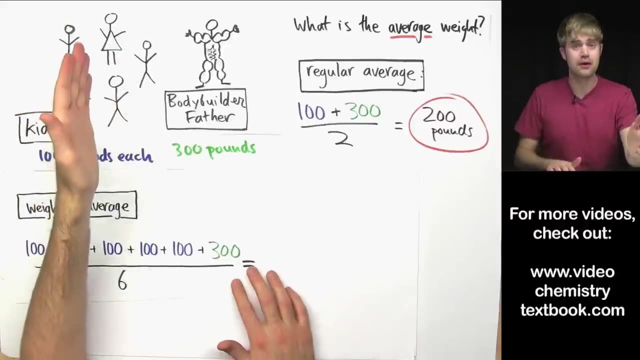 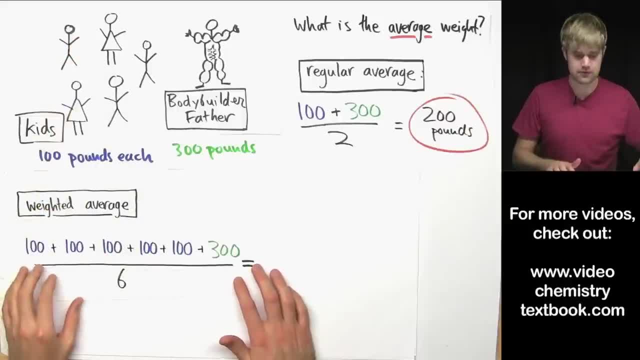 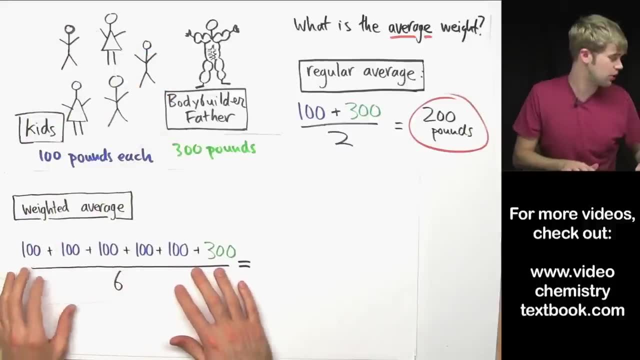 hundreds for each of the kids, for the five kids, and then I add three hundred for the weight of the bodybuilder and then I divide by six, because there are six things total. Sometimes it's easier to express this with multiplication. I've got five times a hundred. 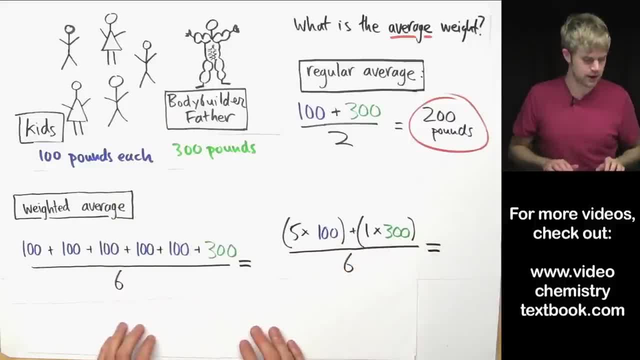 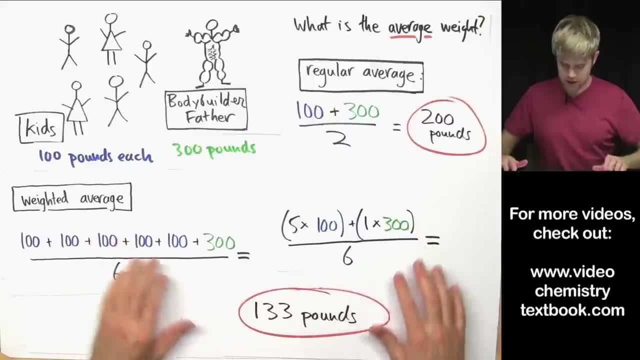 plus one times three hundred divided by six, because there are six things. When we crank through these equations, we end up with a different answer than this. Okay, Okay, We end up with a hundred and thirty-three pounds. This is the answer to the weighted average. 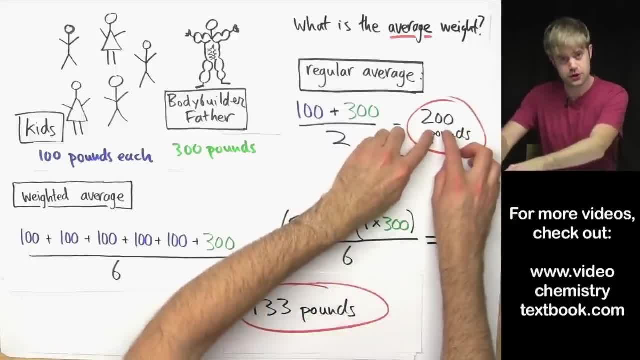 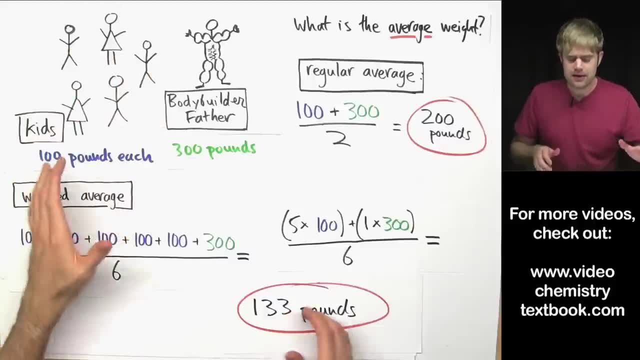 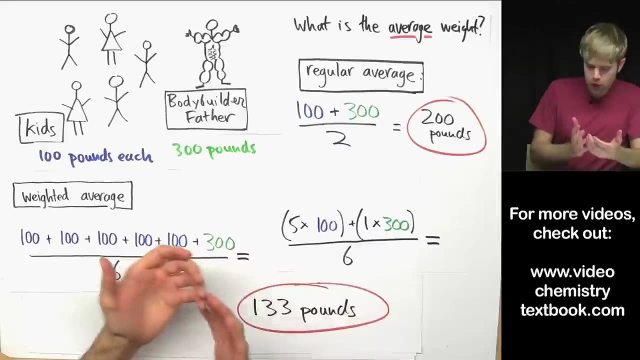 Now you'll notice this number. one hundred thirty-three is much less than two hundred, and one hundred thirty-three is a lot closer to the weight of the kids. That's because of the weighted average and how it works. The weighted average will pull down the average closest to what. 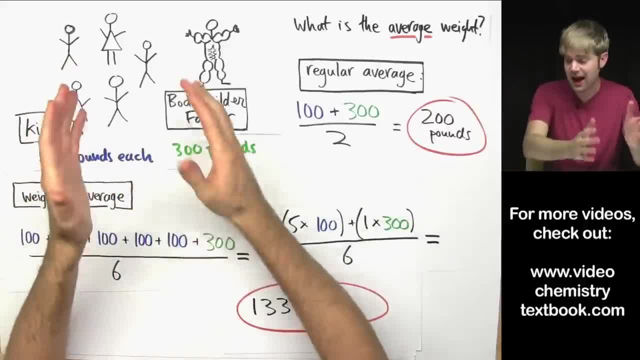 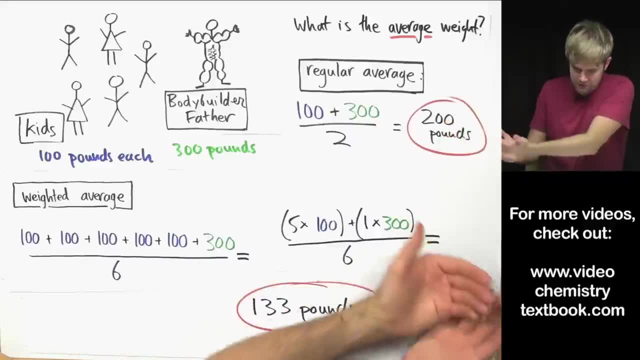 ever we have the most of. Okay, so if it were just half and half, it would be two hundred pounds. we have the same number of each, But since we have more of the kids, we take that two hundred and we pull the number down. 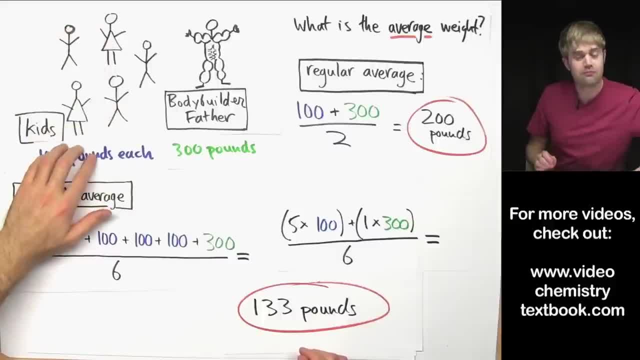 closer to the weight of what we have more of. So that's why the weighted average for here is a hundred and thirty-three, very close to the weight of the kids. Now, the weighted average could work the other way as well. Let's say that we had a group. 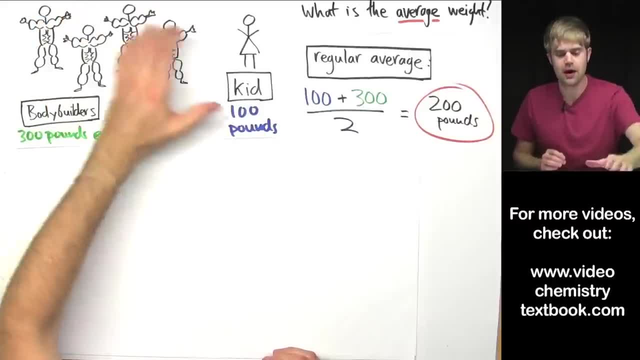 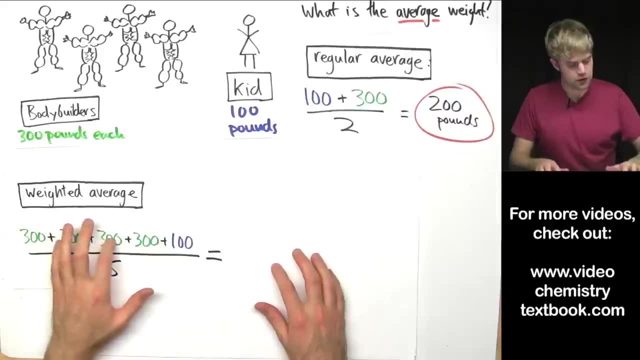 We're four people, we're three hundred pound bodybuilders and there's only one kid that weighed a hundred pounds. In that case we calculate the weighted average: one, two, three, four, three hundred pound bodybuilders plus one one hundred pound kid, divided by five total, or we could do this: 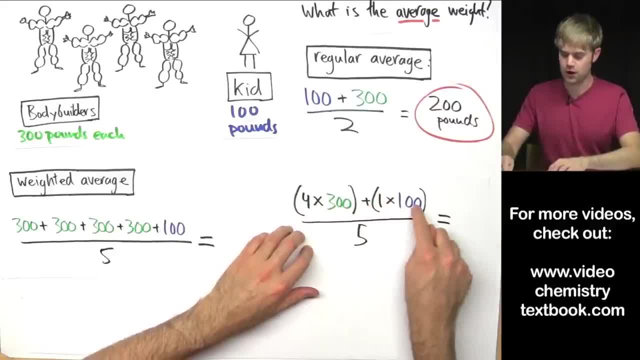 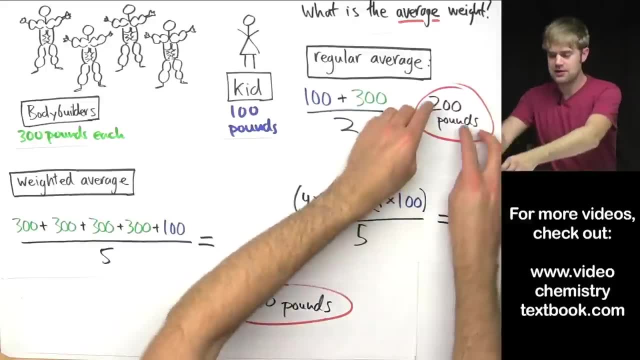 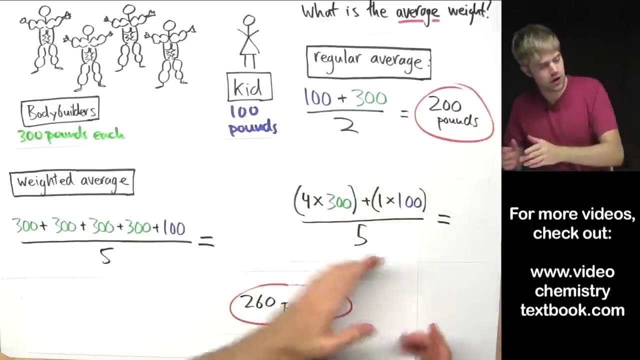 with multiplication parentheses: four times three hundred plus one times one hundred divided by five, And in that case we get two hundred and sixty. All right, This number is a lot higher than the number two hundred. that's right in between, and it's much closer to the weight of the bodybuilders. it's much closer to three hundred because 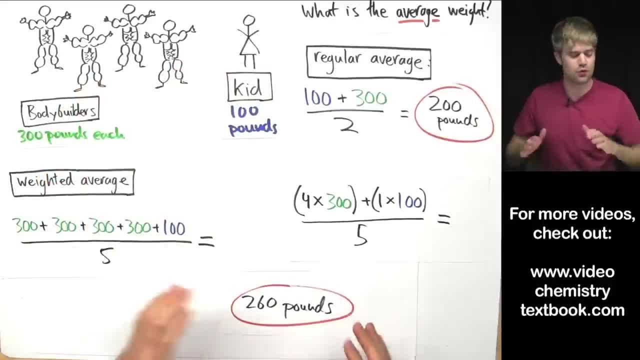 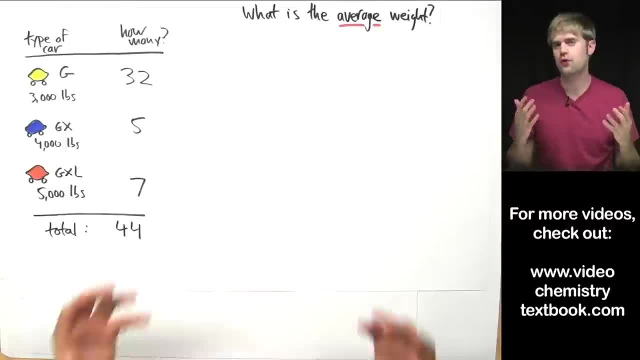 there are more of the bodybuilders. there's only this one kid. So the weighted average should be closer to the weight of what we have more of Now. for a weighted average we don't just have to have two things like the kids and the bodybuilders. 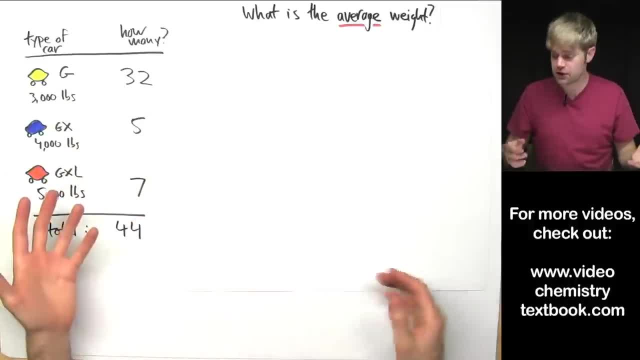 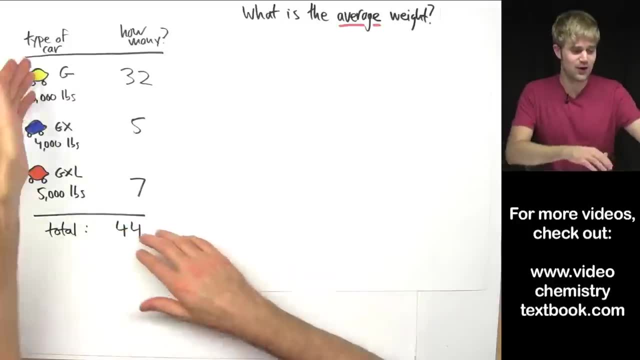 We can have a number of different things. We can have more than two and we can have a whole bunch of them. In this case, I'm talking about a parking lot that has three different kind of cars. They're all called Limonas because they look like a lemon. 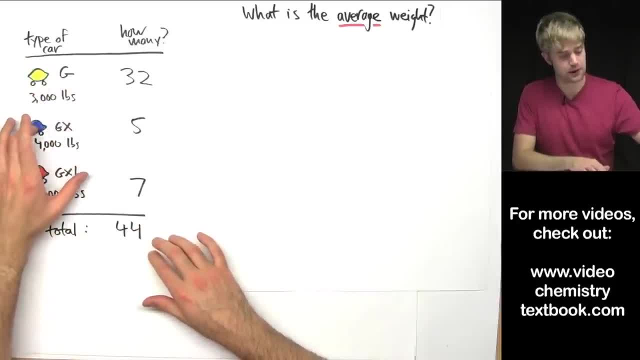 Got the Limona G that weighs three thousand pounds, the Limona GX that weighs four thousand pounds and the Limona GXL, which weighs five thousand pounds, And I have different amounts of each of them. So how would I calculate a weighted average here? 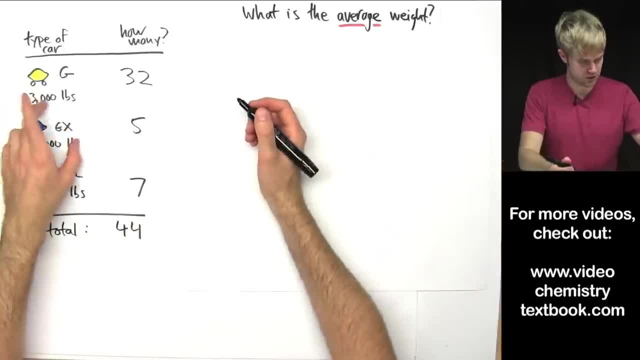 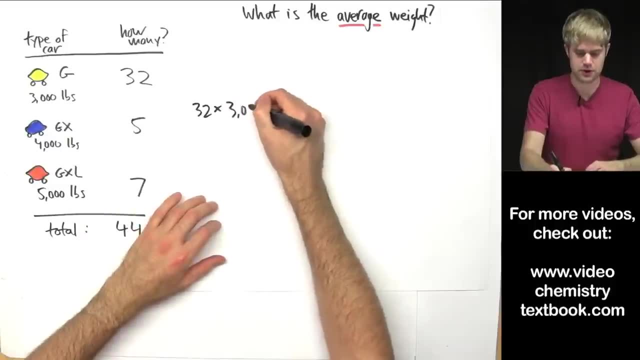 What I do is I take the weight of the Limona G- That's three thousand pounds, Three thousand pounds- and I multiply it by how many Limona Gs there are. They're thirty-two times three thousand pounds each. I take that and then I add the number of GXs. 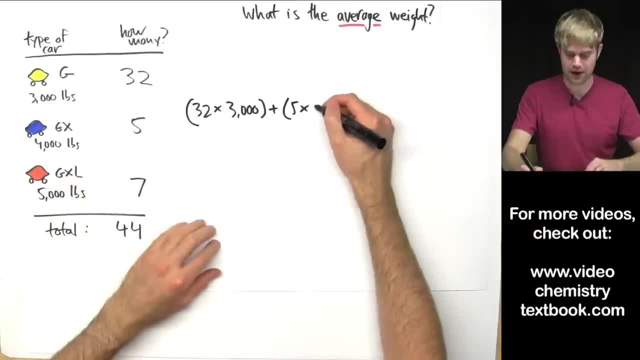 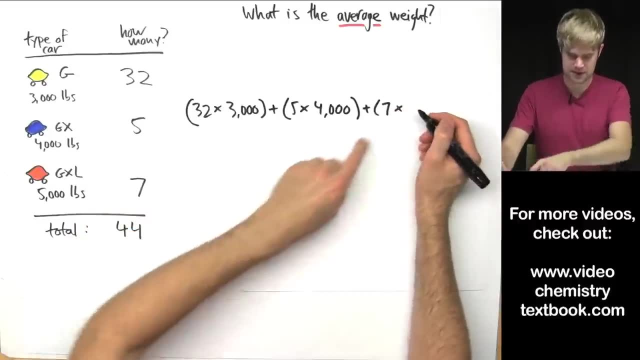 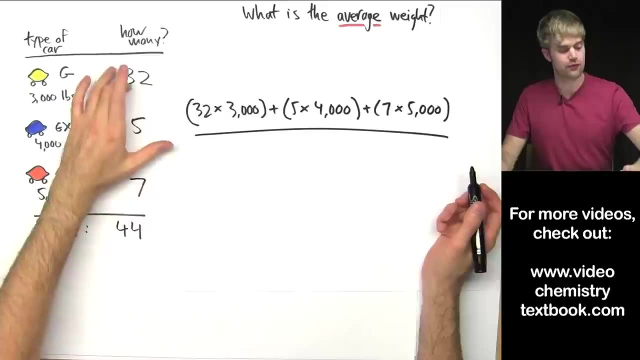 So I've got five of them five times four thousand. And then the GXLs. I've got seven of them plus seven times five thousand pounds. Now I do this, I've accounted for the weights of each one of these cars, and now I've got to divide by. 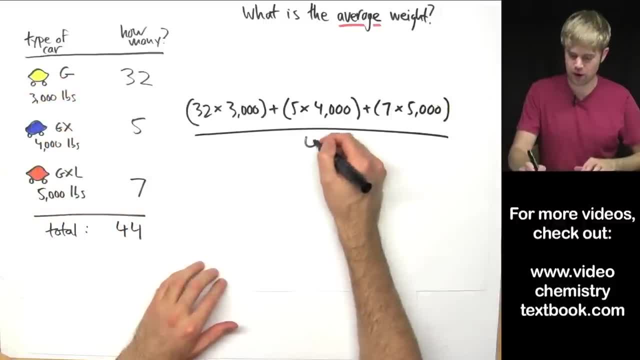 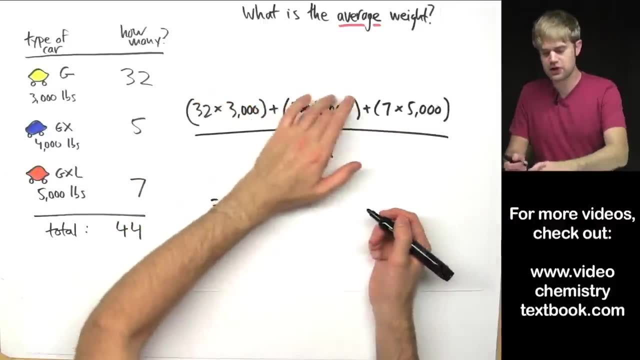 the total number of cars I have in this group, and that's forty-four. So these are the Gs, these are the GXs and these are the GXLs. Do the multiplication of each, add it up, and I'll end up with three thousand four hundred. 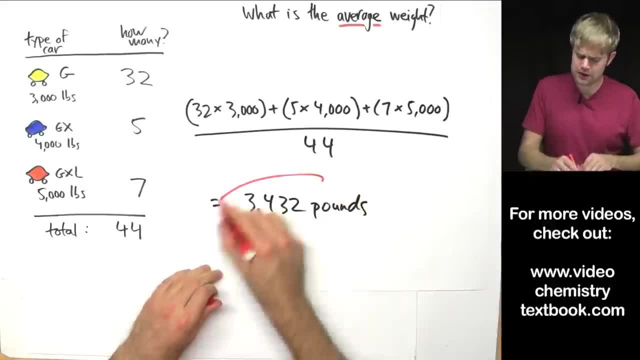 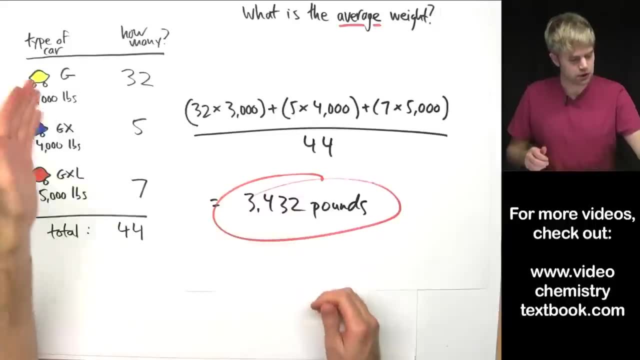 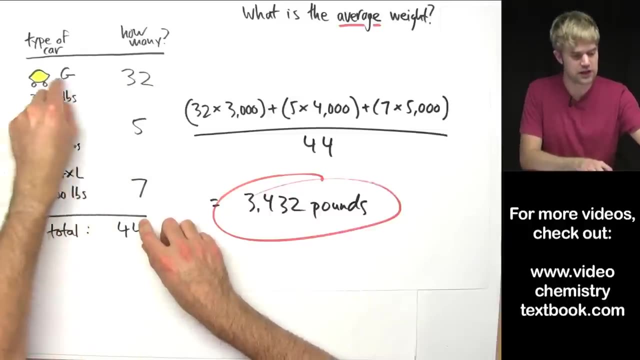 and thirty-two pounds. Now look at how this number compares to the weights of the individual cars. This number is closest to the weight of the G, and that makes sense, because I have a lot more of the Limona Gs than I have of the heavier GXs and GXLs. 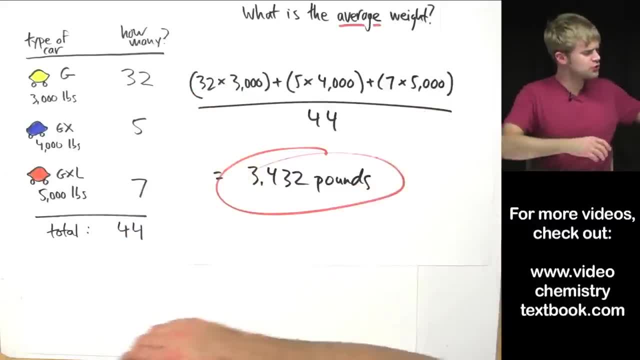 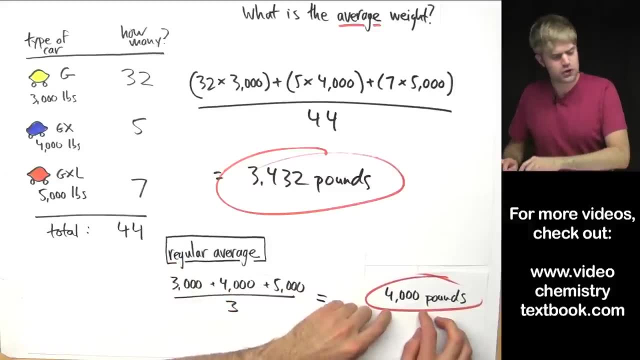 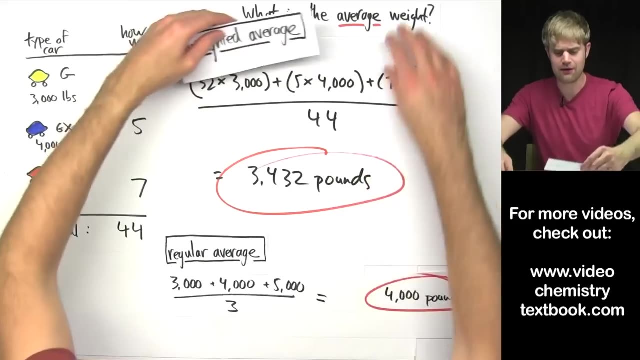 So this is the weighted average, whereas the regular average for these cars would have been three thousand plus four thousand plus five thousand divided by three, which would have given us a number that was smack dab in the middle. But once again, the weighted average here. The weighted average gives us a number that takes into account how many of each type of 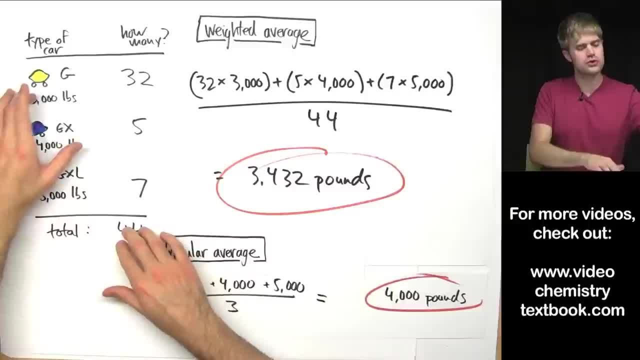 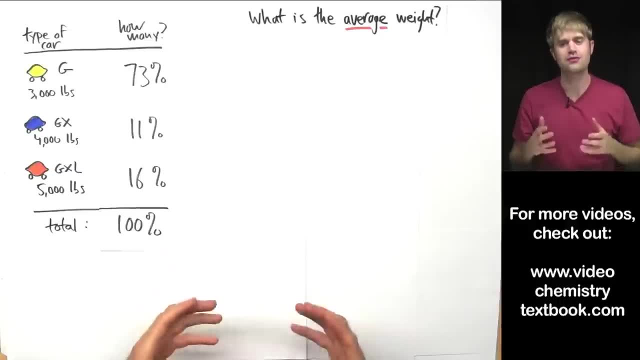 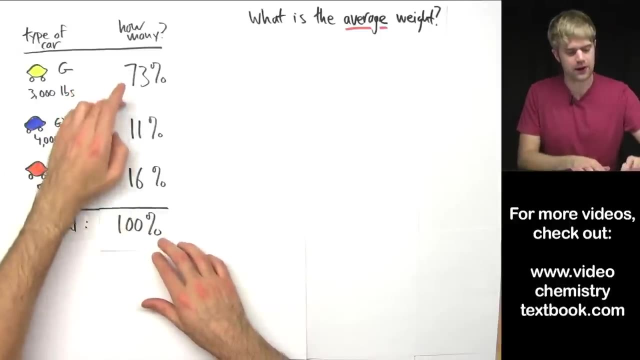 these cars I have and gives me a number that is much closer to the type of car that I have the most of Now, a lot of times when you're talking weighted average, you'll have to work with percents. So instead of getting the number of things, you'll get the percentages of them, like right. 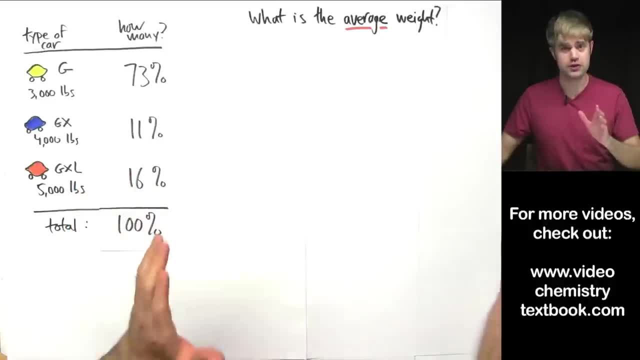 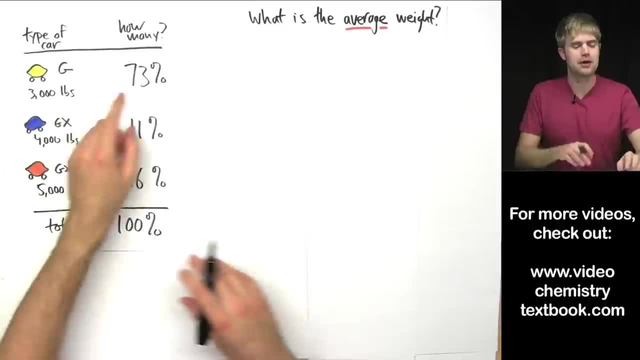 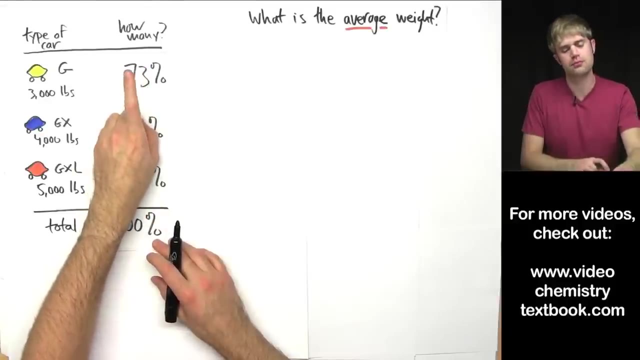 here. Here's how you calculate a weighted average using percents. What I'm going to do is I'm going to take the weight of the Limona G here and I'm going to multiply it by seventy three percent, expressed as a decimal. So the decimal place in seventy three percent would be here: 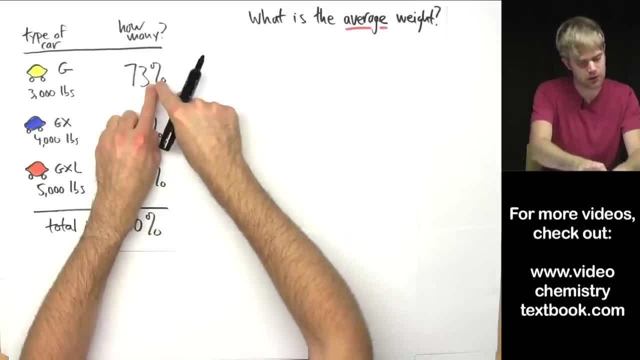 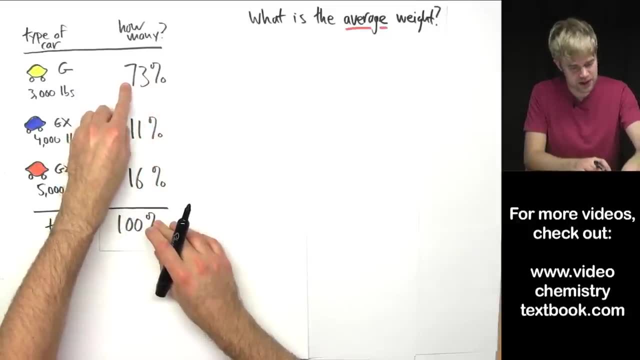 To turn this percentage into a decimal, I have to move the decimal place two spots to the left, So I'm going to move it to here. to here. The decimal place is going to end up right here, So I'm going to do. 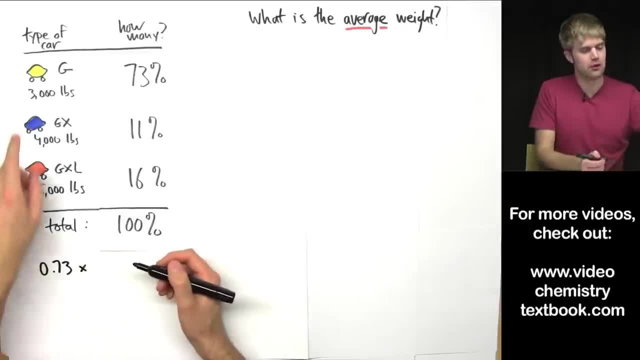 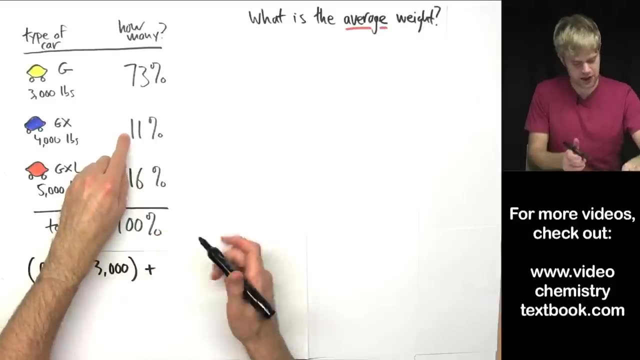 Zero point Seven, three, And then multiply that times the weight, Three thousand pounds. That's the Limona G. Now for the GX, I'll take eleven percent and express that as a decimal. Move the decimal place two spots to the left. so it's going to end up here. 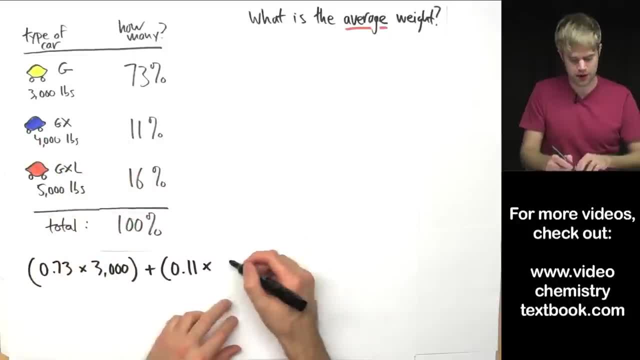 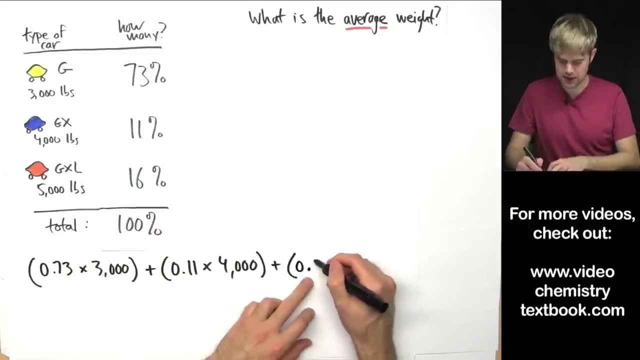 Zero point one one And multiply that times the weight of the GX- Four thousand pounds for that model of the car. And finally, I'll take sixteen percent and express it as a decimal Zero point one six And multiply it by the weight of the GXL model. 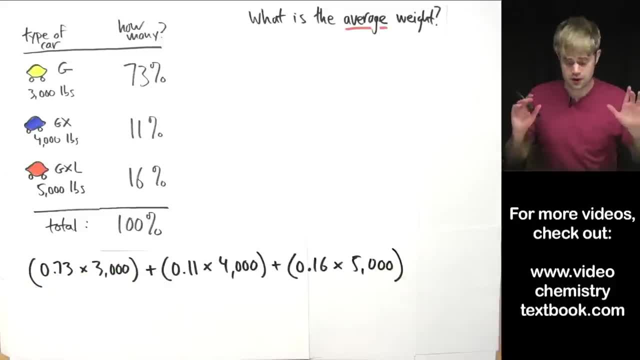 Now, when you're working with percentages, you don't divide by anything. All you do is multiply the weights by the percentages expressed in decimals, and that's all you have to do. This is the same problem as the one that I did before. We're just expressing these abundances, or the amount that we have, in percents, so the 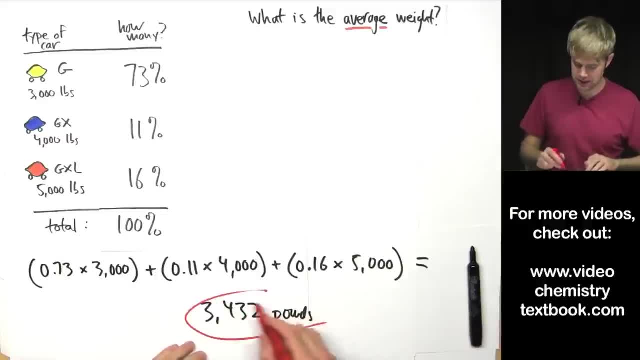 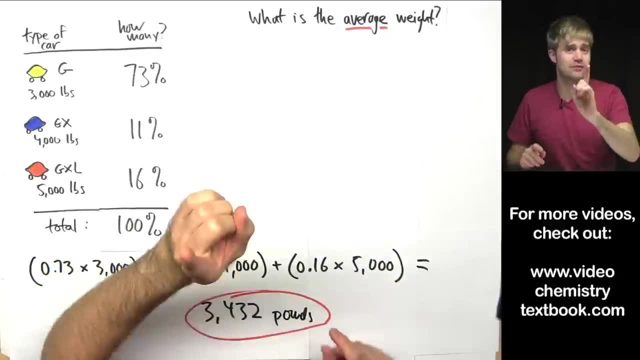 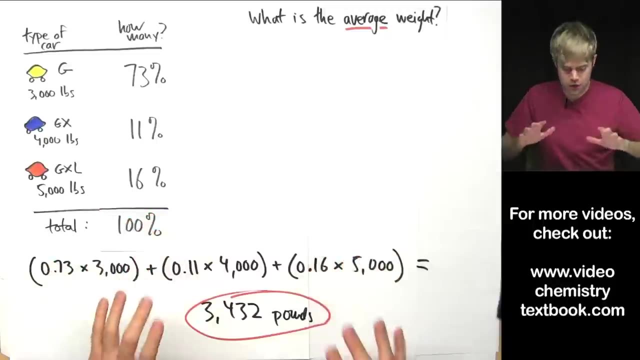 answer: Four hundred thirty two pounds is going to be the same as what we got earlier. Anyway, that's how you do weighted average using percents. Now I have to say this: Weighted average doesn't mean that you have to use weights of things. 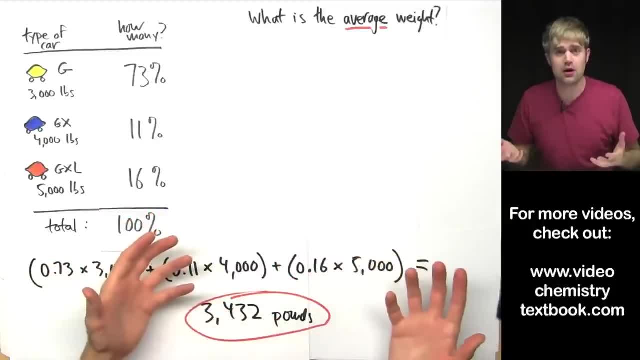 You can calculate a weighted average with the amount of money people make, or like how much volume you have in different types of containers. Anything you can think of, Any measurement you can think of, You can do a weighted average of. So I've been using examples of weights here. 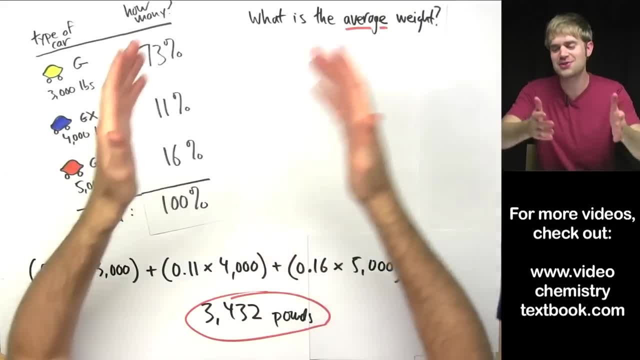 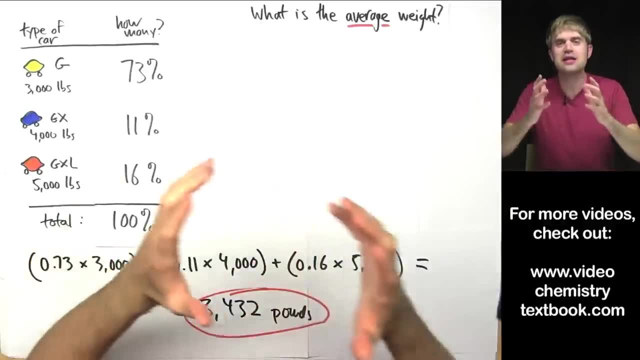 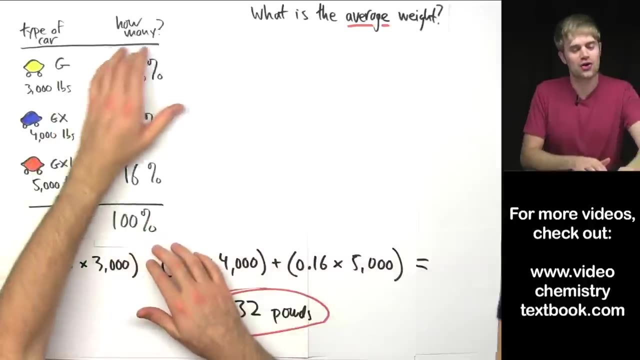 Weights of people, Weights of cars, But you don't just have to do weights for a weighted average. The only reason you call it a weighted average is because it takes into account the number of each thing you have, and they kind of pull the average closest to their value. 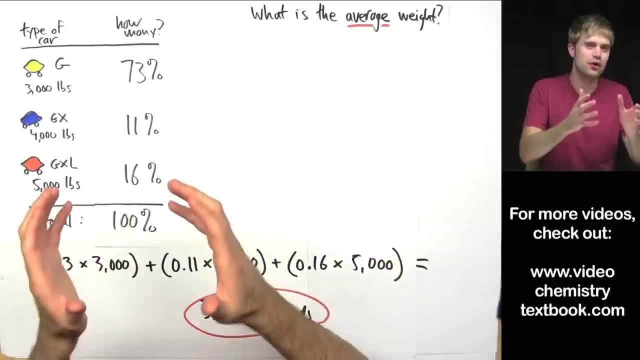 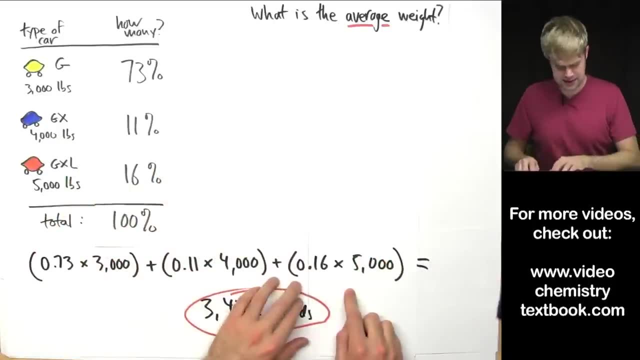 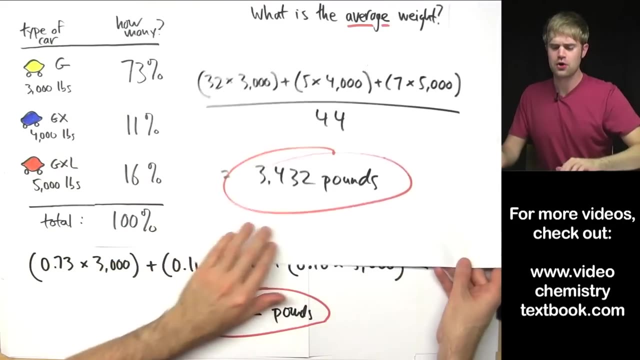 So that's why you call it a weighted average, Because you give different weight Weight to each type of thing that you have. Finally, if you're interested to see how this equation here is the same as the one that I did here, you can finish this video up. 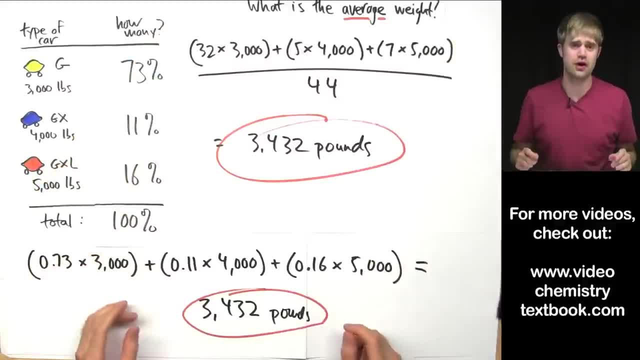 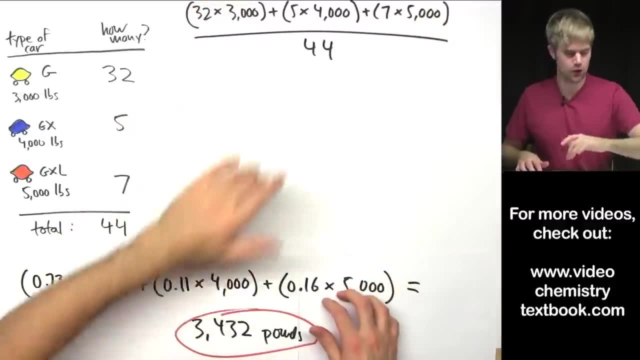 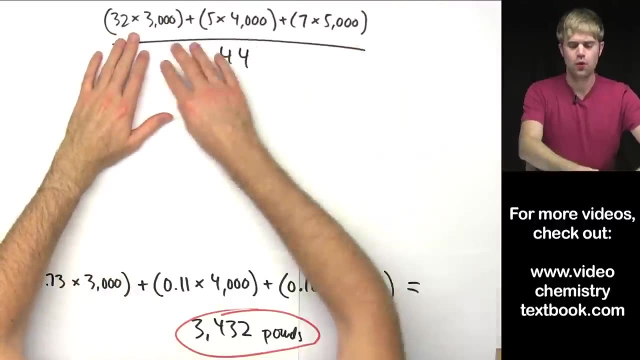 I'll show you at the very end how these are equivalent expressions. So these two expressions are equivalent ways of writing the calculation for the weighted average for this information here. Let me show you. Let me show you how they're equivalent. We're going to take this and we want to end up with something that looks like this: 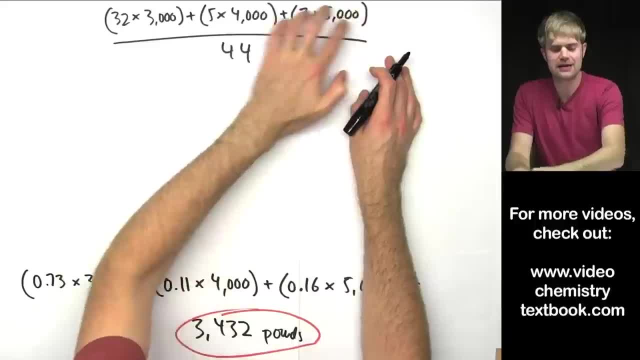 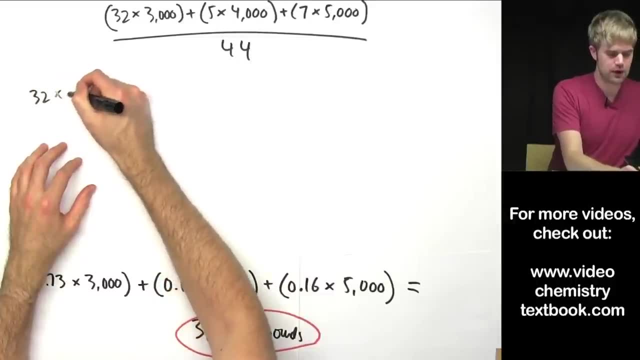 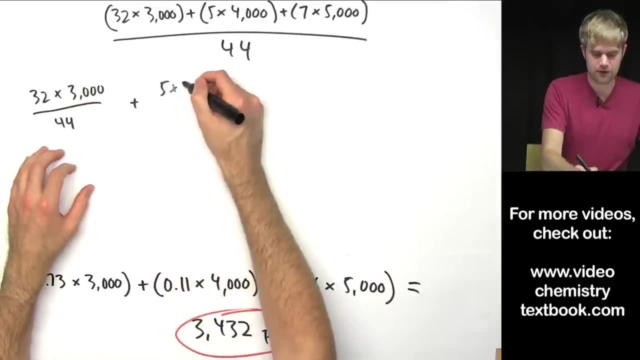 The first thing we can do is we can see these three different things that are added together on the top of a fraction. We can separate them out. So I'm going to do thirty-two times three thousand divided by forty-four, plus five times four thousand divided by forty-four.